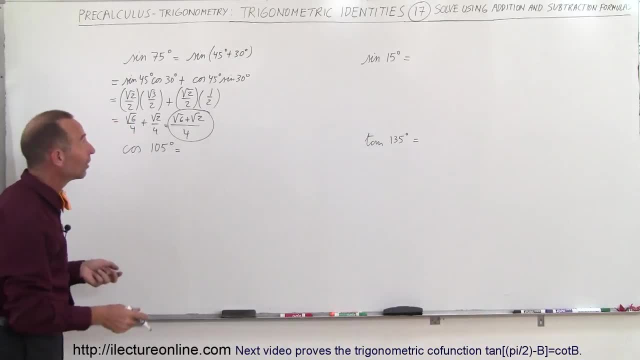 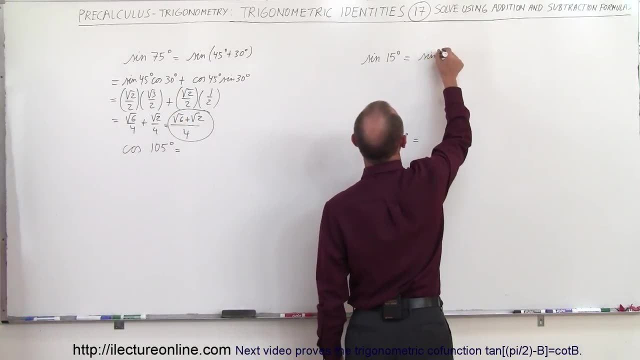 And so you can see that that is pretty easy to do using the addition formula. Let's try the same for the sine of 15 degrees. This can be written as the sine of 45.. This can be written as the sine of 45 degrees minus 30 degrees. 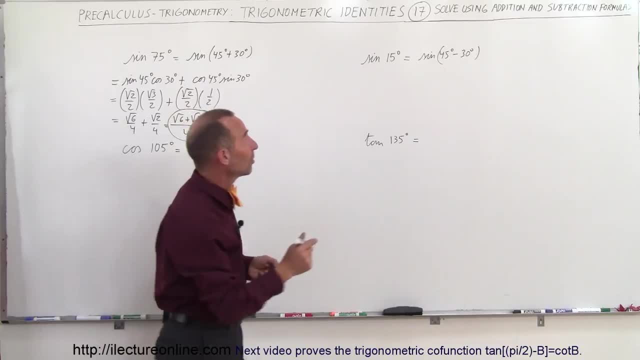 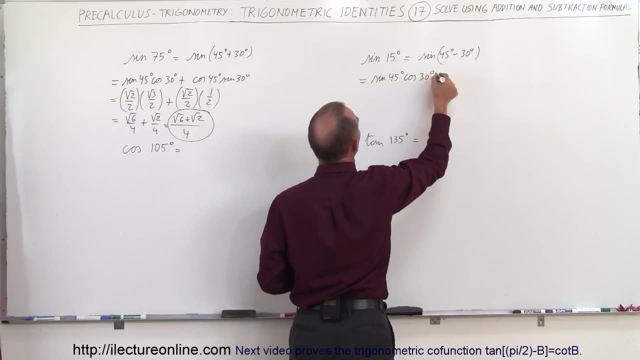 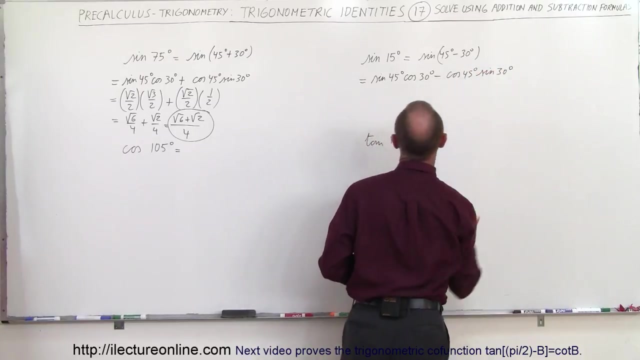 And so now we have the sine of the subtraction of two angles. This can be written as: the sine of the first angle times the cosine of the second angle, minus the cosine of the first angle times the sine of the second angle. The sine of 45 degrees is square root of 2 over 2.. 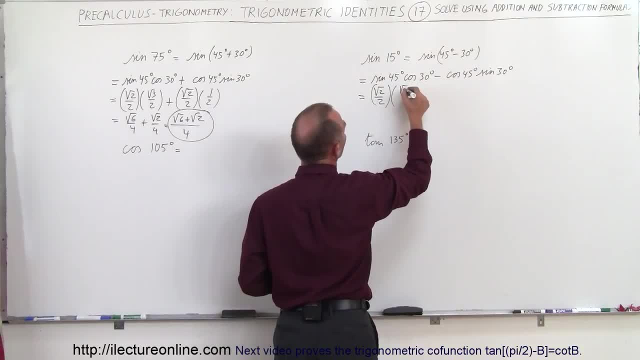 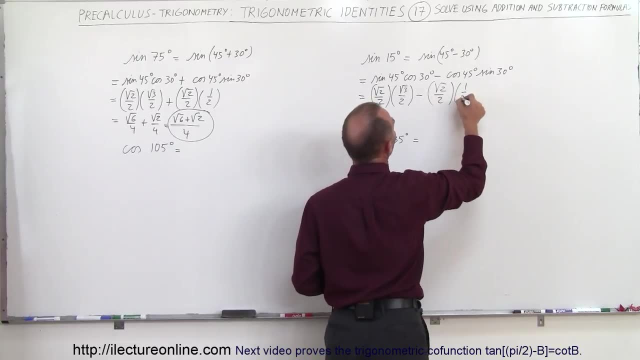 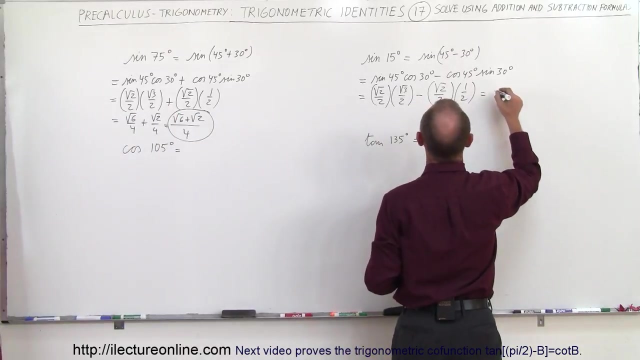 The cosine of 30 degrees is the square root of 3 over 2.. minus the square root of 2 over 2 times 1 half, and so it's kind of the same as what we had over there, except we have a minus instead of a plus. so this becomes equal to the square root of 6 over 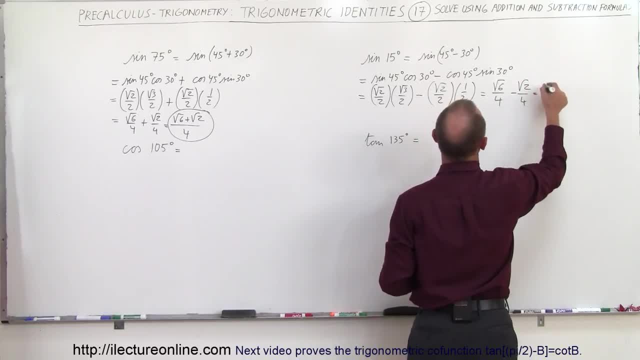 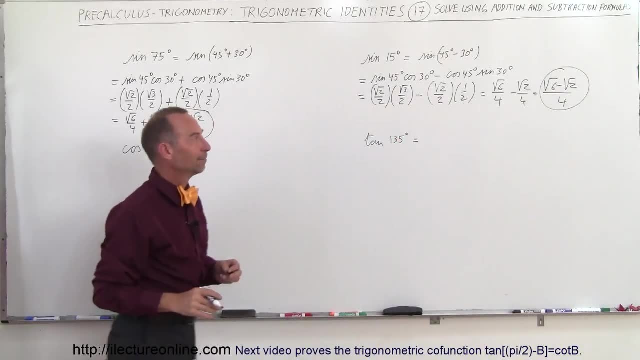 4 minus the square root of 2 over 4, which is equal to the square root of 6 minus the square root of 2, all divided by 4, and so that would be the solution for that, The cosine of 105 degrees. let's see here: 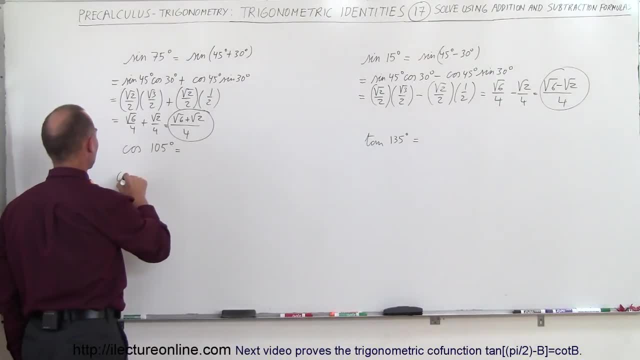 we can make that 60 plus 45, so we have the cosine of 60 degrees plus 45 degrees. so how do you write that? well, it's the sum of two angles for a cosine. that means it's the cosine of the first angle times the cosine of the second angle, and if we have a plus there that becomes minus the sine of. 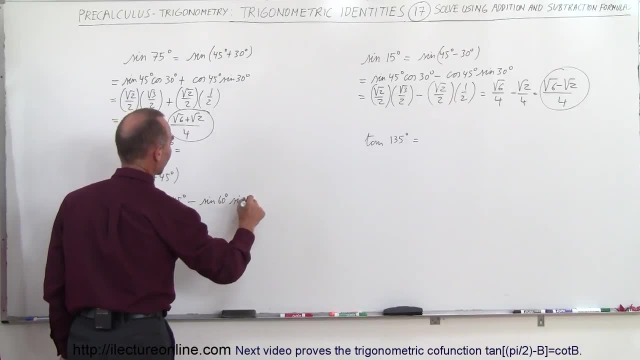 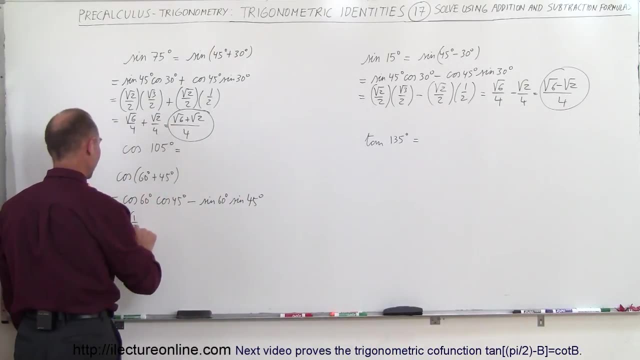 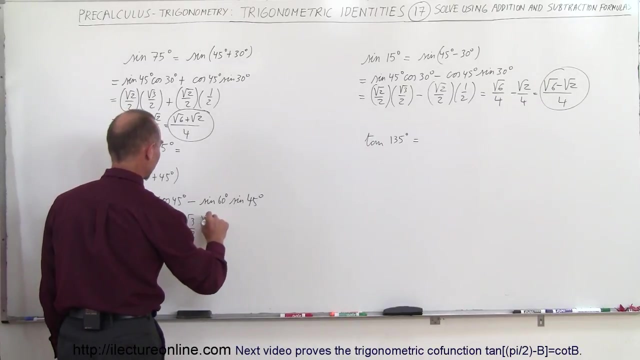 the first angle times the sine of the second angle. the second angle is 45 degrees. All right, so this becomes one half times the square root of 2 over 2 minus. that would be the square root of 3 over 2 times the square root of 2 over 2. so this becomes equal to the square root of 2 over 4 minus the square root. 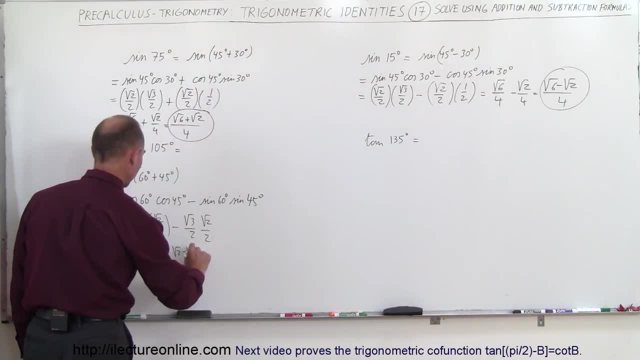 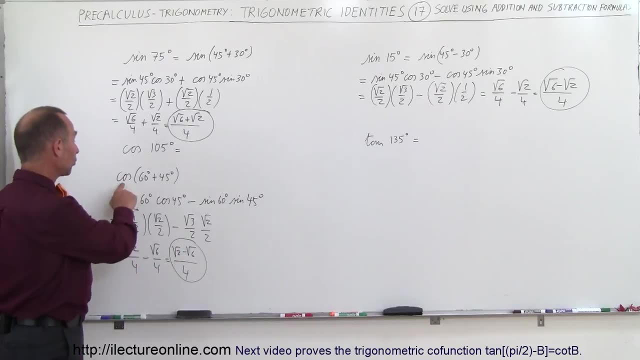 of 6 over 4, which is equal to square root of 2 minus square root of 6 over 4, and so that would be the solution there. Now, that makes sense that that would be a negative number, because the cosine of an angle bigger than 9 degrees is indeed a negative number. and finally, the tangent of the 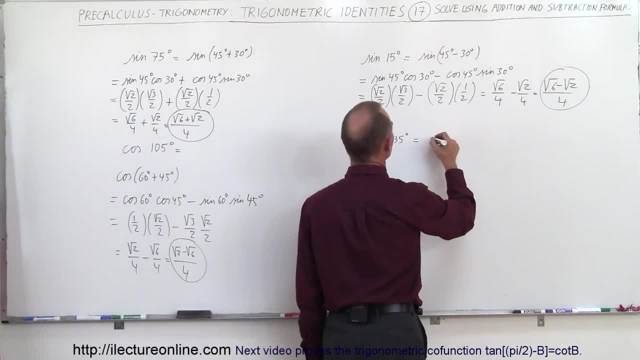 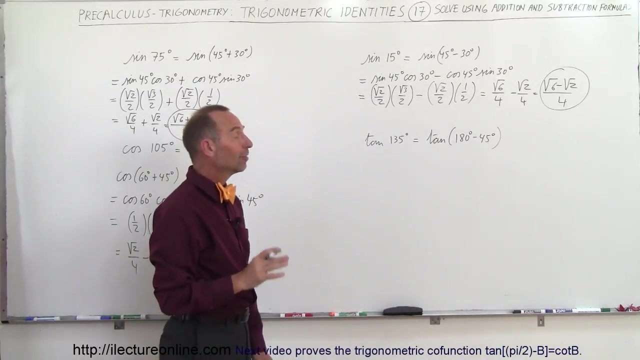 of 135 degrees. why do you say that could be the tangent? Let's see here. How about the tangent of 180 degrees minus 45 degrees? All right, It's better to do that than to go. the tangent of 90 degrees plus 45 degrees, because the tangent of 90 degrees, that's. 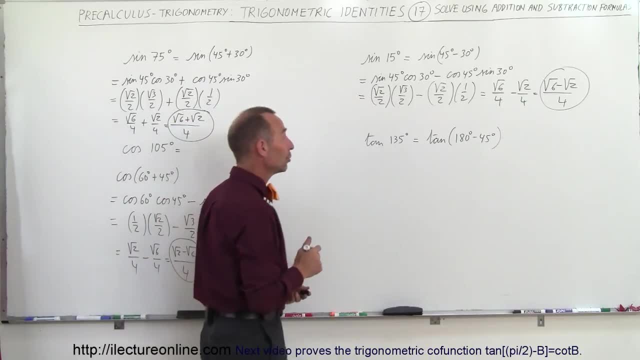 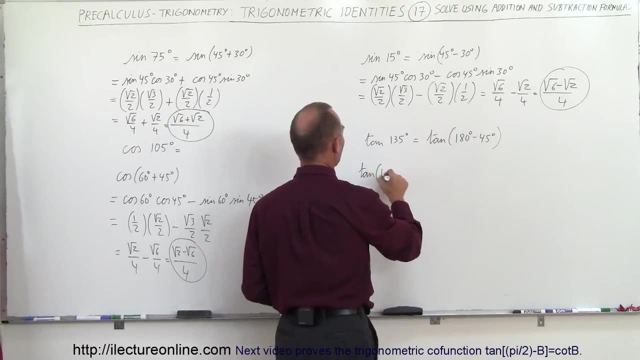 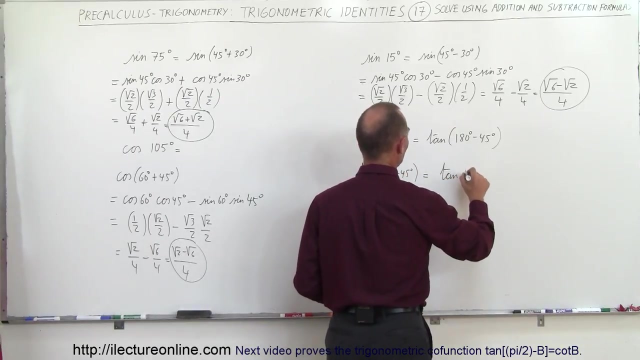 infinity, And so you couldn't solve it that way. So you have to be careful here what you do. So we can say that's equal to: so the tangent of 180 degrees minus 45 degrees, that is equal to the tangent of the first angle, 180 degrees minus the tangent of the second. 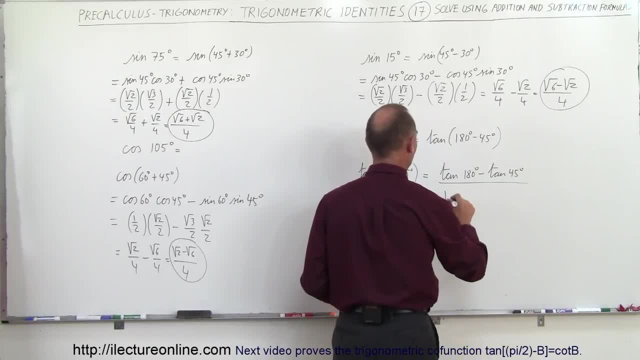 angle: 45 degrees, all divided by 1, plus the tangent of the first angle times the tangent of the second angle. All right, So let's see what that ends up doing. So what that ends up being the tangent of 180 degrees is the sine over the cosine, and 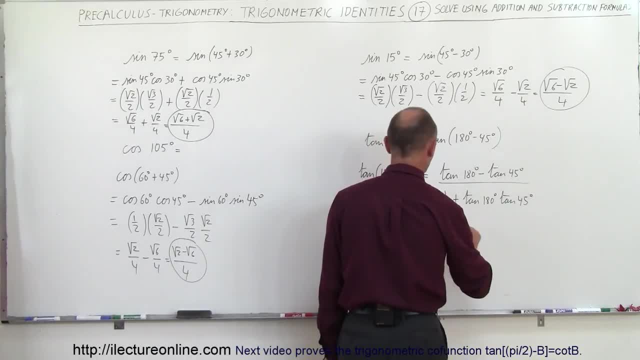 the sine of 180 degrees, that's 0.. So this would be 0 minus, and the tangent of 45 degrees is equal to 1.. So that would be 1 divided by 1 plus the tangent of 180 degrees, That's. 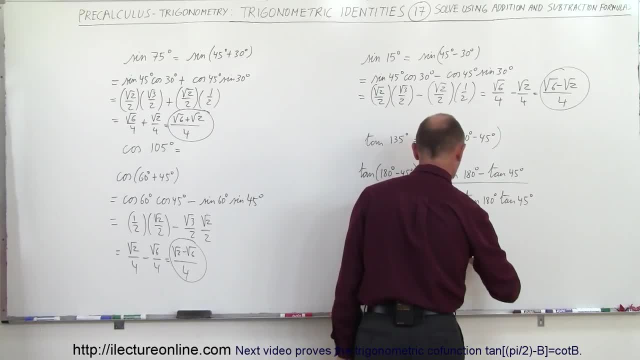 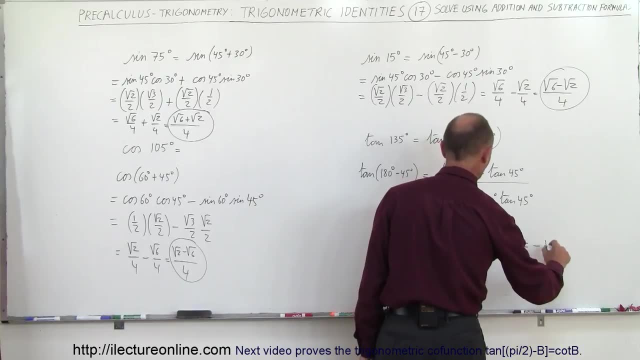 equal to. let's see here that would be 0 times the tangent of 45 degrees is 1.. So it would be equal to minus 1 divided by 1, which is minus 1.. And that's the answer there. So 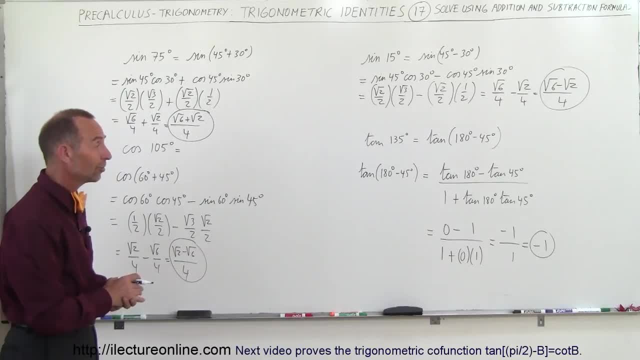 you could see that Using these addition and subtraction formulas, you can very easily find the sine of the cosine or the tangent, or something like that, of some unusual angles that otherwise you'd need to grab a calculator to solve. But here you can do it just like that.